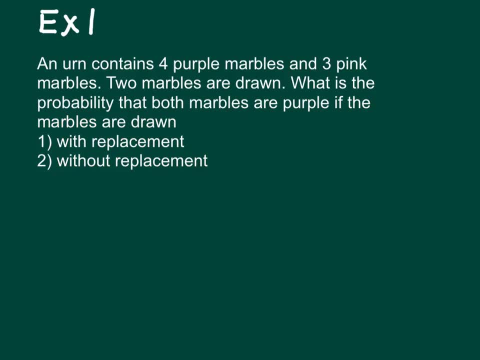 Now, the problem that I just went over was called probability with replacement, because we replace the marble that we drew. Now let's take a look at this example. It says an urn contains four purple marbles and three pink marbles. So in other words, 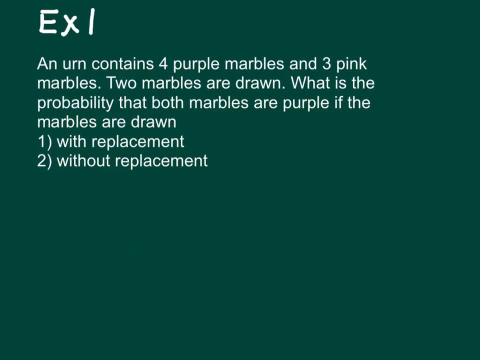 there's seven marbles in the urn. It says two marbles are drawn. So in other words, I take a marble out, I look at the color, I take another marble out and look at the color. Now it says: what's the probability that both marbles are purple if the 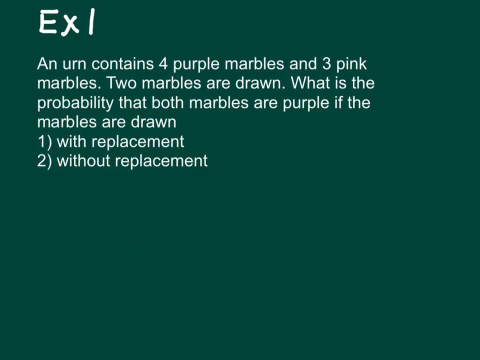 marbles are drawn, Number one with replacement And then number two without replacement. Now, here is this. this is what this means. Let's talk about the, the with replacement first. So, in other words, I'm going to take a marble out, I'm going to look at the. 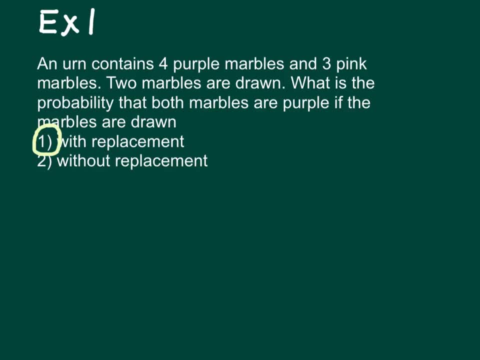 color and then I'm going to place it back into the urn. So we're still seven marbles. Then I'm going to draw another marble out and look at the color and then put it back. So this is what we call with replacement, And we want to know what's the. 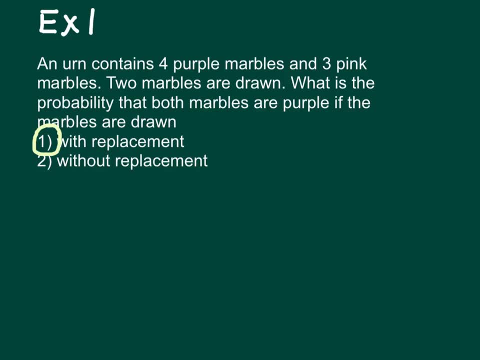 probability that both marbles are purple. Well, all right, let's let's look at number the first part of this. So I'm going to take a marble out. What's the probability it's going to be purple? Well, there are four purple out of a total of seven marbles. right, So I take a marble out. 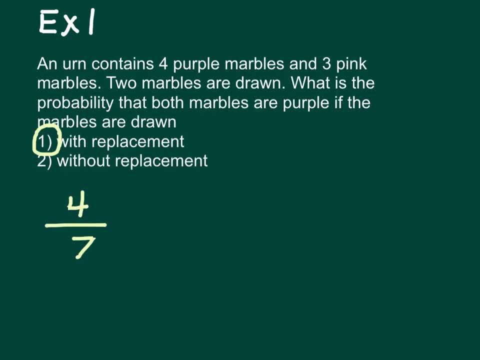 I look at it, the probability it's purple is four out of seven. I put the marble back. Now I'm going to draw a second marble. What's the probability that the second marble is purple? Well, there's still seven marbles in there right, And there still could be four purple marbles in there. 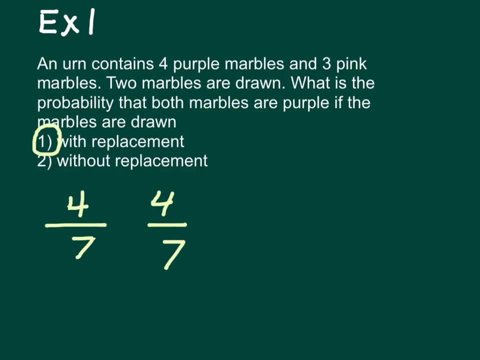 because I replaced that first one. right Now I've got two different situations here, right. So I want to know that the probability that I draw and the first one's purple, I replace it, I draw again and the second marble's purple, So I multiply these two events or drawings together. 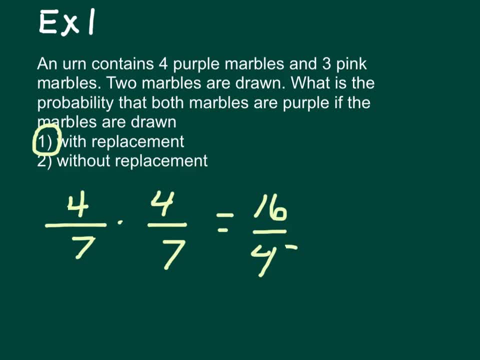 So four times four is 16, and then seven times seven is 49. So the probability with replacement is 16 out of 49. Now that's what we call with replacement. all right, Now let's take a look at what happens when we do that. So let's take a look at what happens when we do that. 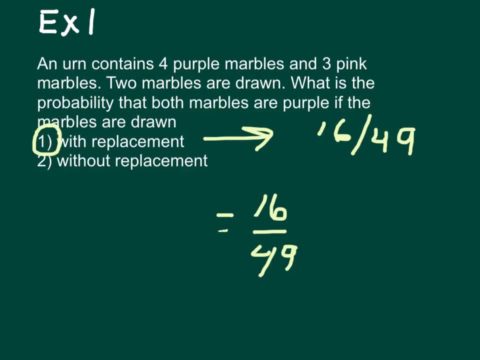 What happens in number two if I don't replace the marble? So, in other words, let's talk about this. So, in other words, what's the probability? I draw two marbles and they're both purple, but I don't replace that first marble. All right, so I've got this jar. I'm going to pick out a. 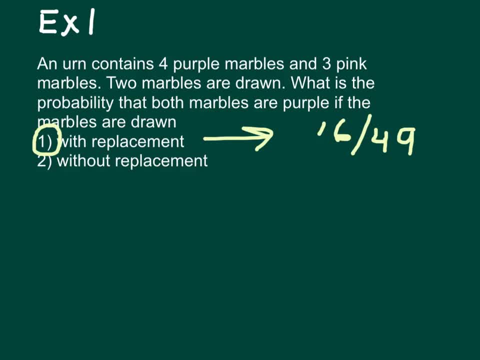 marble. So I pick a marble out, I look at the color. What's the probability that it is purple? Well, same as before. there were four purple out of seven marbles. But now I don't replace that marble that I just drew out. So I don't replace it. I set it to the 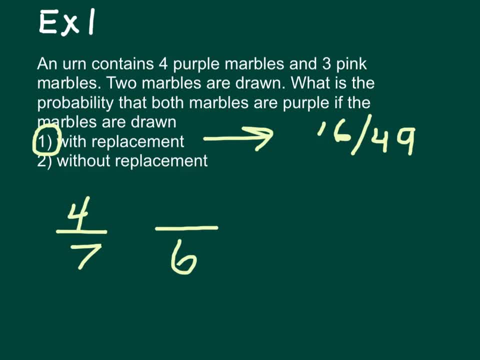 side, which now means that there are six marbles left. all right, Now the probability that that one is purple, So I'm going to so say. I drew that first one out and it was purple, all right. And again we're talking about the chances that the color is purple, So now I don't replace it, Say I. 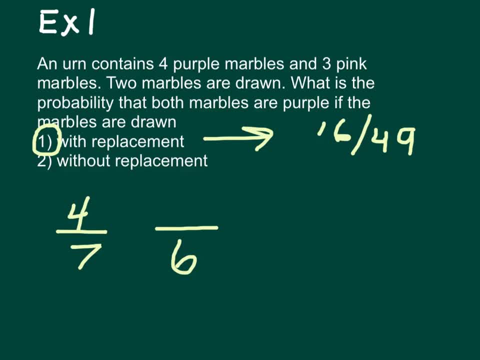 don't replace that purple. And how many purple marbles are left then? Well, there would be three purple marbles out of the six right, Because the first one I'm saying that I picked out is purple. Now I multiply the events. 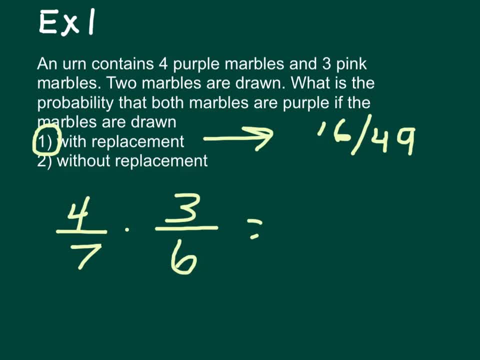 together, I could reduce three over six, you know, if you wanted to, and take four sevenths times one half. That's up to you. So, in other words, multiply them together and you can do some cross-canceling. In fact, that's what I'm going to do. 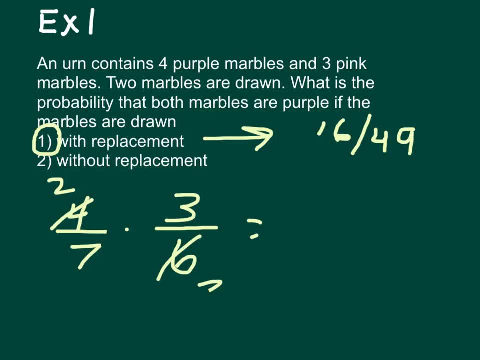 here, So I can divide both these by two, And then three over three is one. Or in other words, let's see: multiply across, I get six over 21. Reduce that, I can divide those by three and I get two. 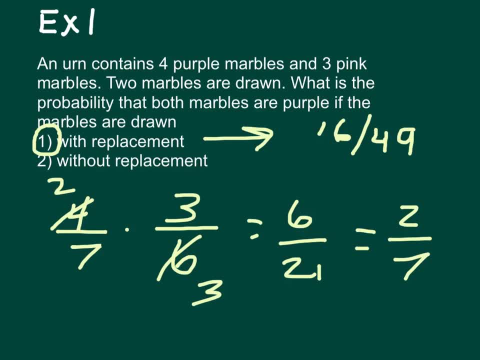 out of seven. So the chances that both of them are purple would be two out of seven, whereas the chances that both are purple would be two out of seven. So I can divide both of them by two and I get purple Without replacement. then would be six out of 49.. So these are the two ways here that 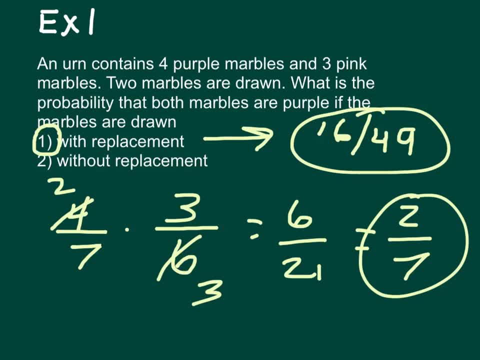 I could do this- And this is called probability- without replacement.